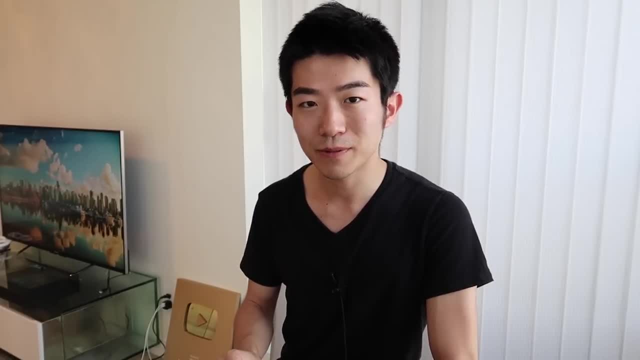 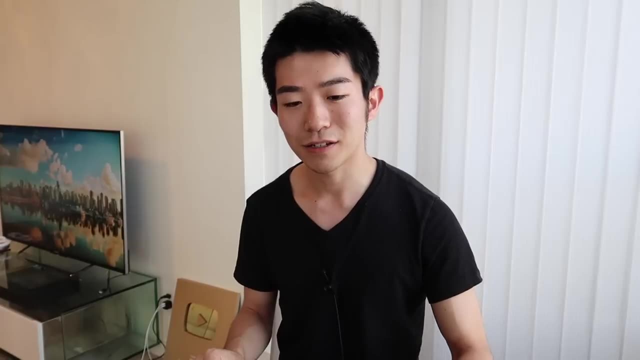 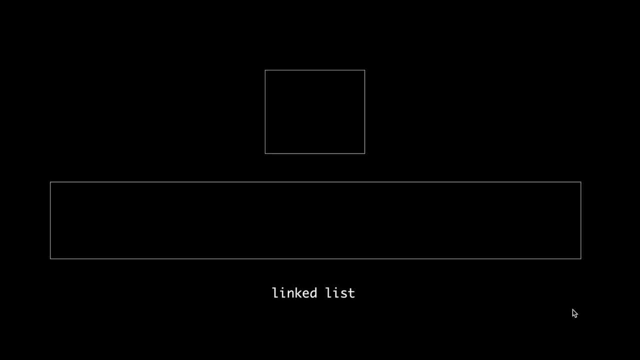 Hey everyone. In my last few videos I made a Q&A website for coders and I still work on it from time to time, But in this video I decided to switch topics and restart my data structures and algorithms series Now, in a previous video which I published a long time ago, we learned the linkless data structure. 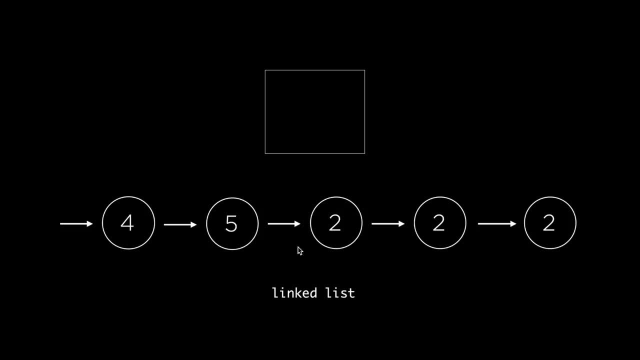 It looked like this one, where we had a bunch of nodes that are connected to each other in a single direction And each node in the structure had a class. like this: It's called node and it has two attributes: integer data and next, which is also a node, 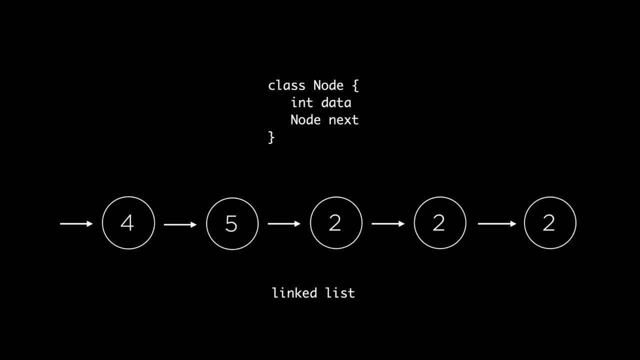 Now, a tree is a similar data structure to a linked list, And the only difference is that in a linked list, each node can only link to one other node, But in a tree, each node can link to multiple other nodes. So here's one example of a tree. 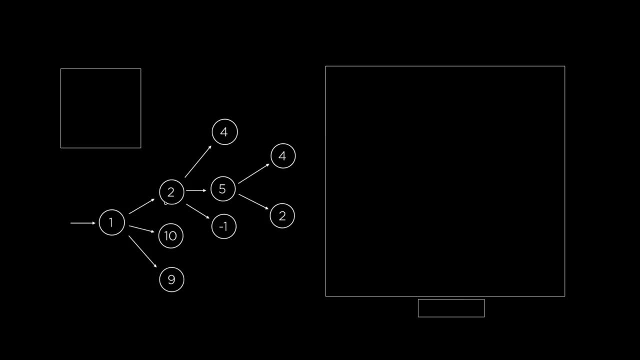 As you can see, each node is linked to one other node. Each node here is linked to multiple nodes. Here each node is linked to at least three other nodes, And so, for this particular structure, the class of each node might look like this one: 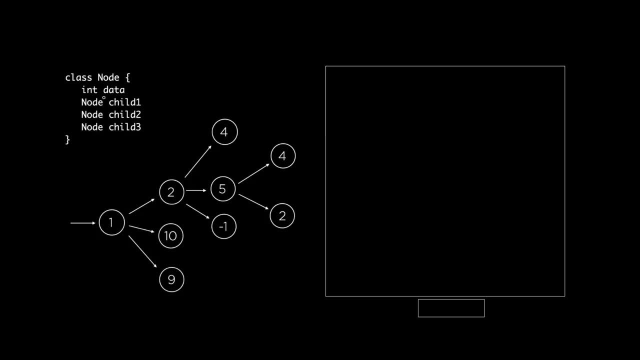 As you can see, this one is called node again and it has four attributes: integer data, just like before. Sometimes this one is called value, but we're calling data here And we have three children. All of them are nodes. 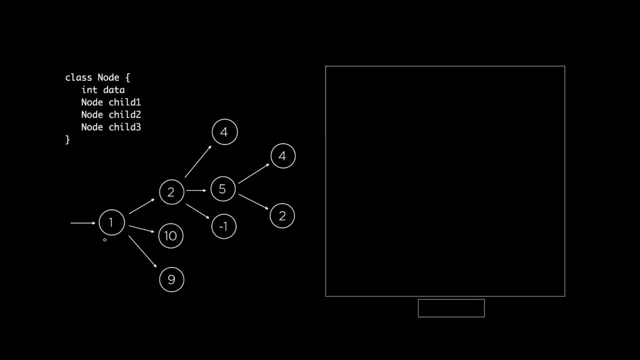 And so, for example, if you look at this particular node here, the three children are set to these three other nodes, And if you look at this node right here, this one has only two children, this one and this one. So if you want to express that in code, you can just set the two of the children to those nodes and the last child to null or none. 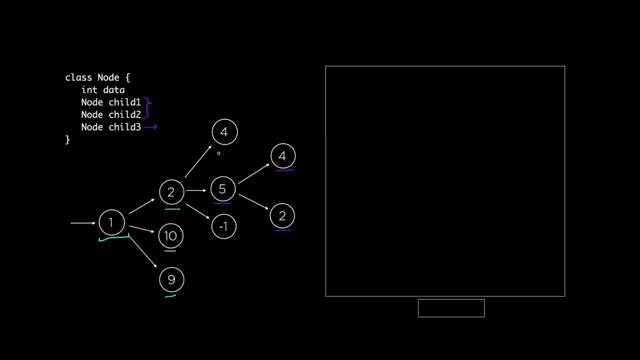 To show that it doesn't exist. And if you look at this node, it doesn't have any children. So you can set all of these children nodes to null or none, depending on the language that you're using. Now let's take a look at another example of a tree. 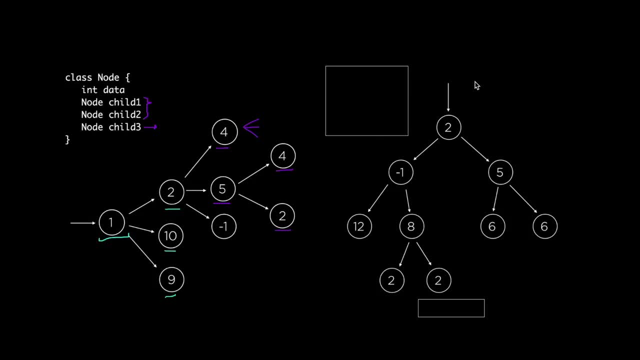 So this one is drawn from top to bottom instead of left to right, But it has the same kind of structure. The more important difference is this one. The more important difference is that each node has at most two children here, So the class of each node might look like this one instead. 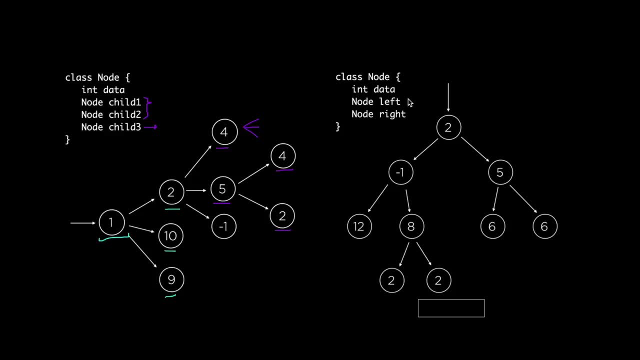 As you can see, we have integer data, just like before, But now we have only two children which we're calling left and right And, just like this, when a tree has at most two children, it's called a binary tree. Now, to help you understand what a tree is exactly, 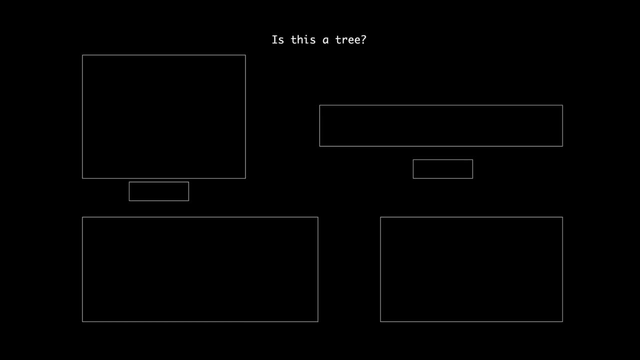 I'm going to call this little game called: Is This a Tree? Basically, I'm going to show you a structure. You just need to answer if it's a tree or not. So let me start with this one. This one doesn't have integers inside them. 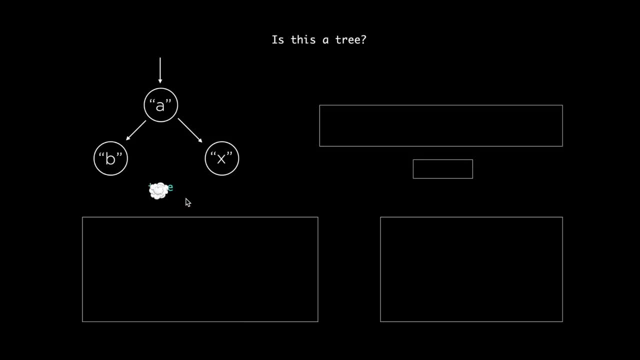 Instead it has strings, But of course it's still a tree. And what about this one? Well, it's a linked list, but it's also a tree, And the way I think about it is that each node could have multiple children, just like that. 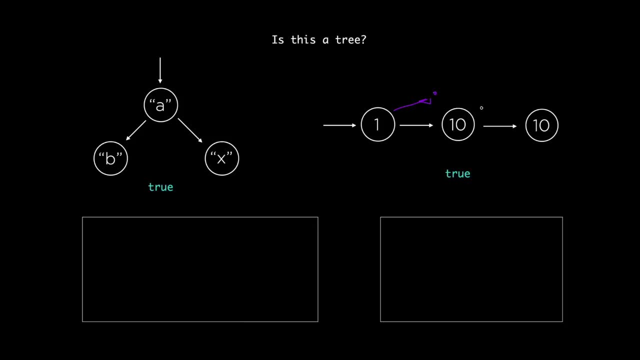 But it just doesn't. So it's kind of a boring example. But technically speaking, it's also a tree. And what about this one? Well, it might look like a tree, but it's not, Because one constraint of something being a tree 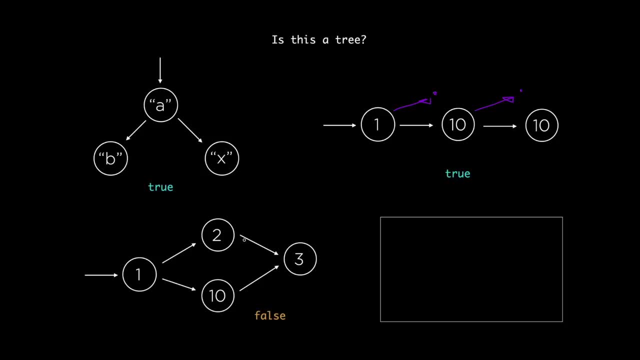 is that there are no two references that link to the same node, And these two references violate that condition. And what about this last one? Well, again, it violates the definition of something being a tree. for the same reason, These two references point to the same node. 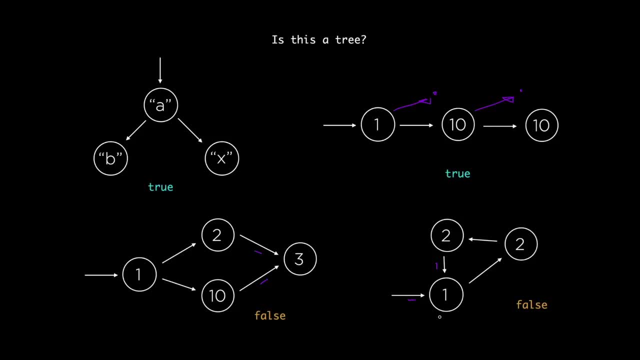 So it's not a tree. And another way to see that this is not a tree is that it has a cycle. here And whenever there's a cycle, that's not a tree. So you might say: well, what is a tree exactly then? 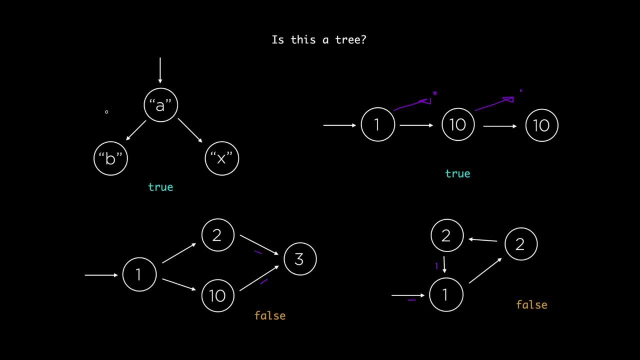 Well, a tree is a structure in which there are nodes that are connected to each other And there's a way to go from the root node to every other node in the structure. So the root node in this particular tree is this one, And there's a way for us to get to every other node. 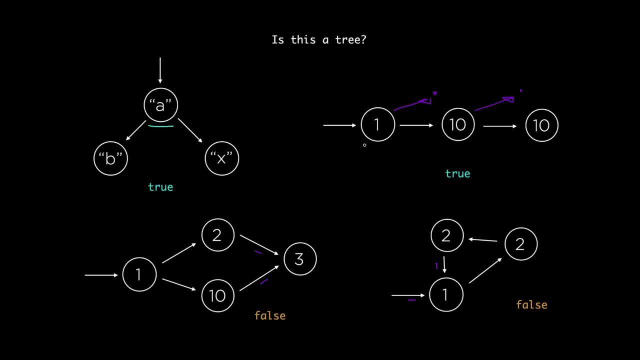 from the root node in this structure And it's the same thing with this tree or this linked list. There is this root node and there is a way to get to every other node from the root node, But as soon as there are two references in this structure, 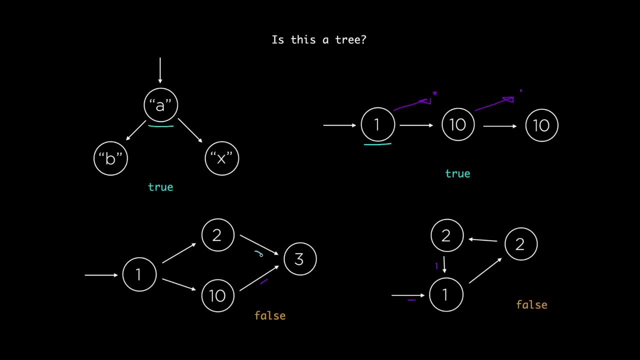 that refer to the same node, for example this one, then it's not a tree anymore. So that's basically what a tree is. And, by the way, the root node of a tree is a node without any parents. So what that means is that whatever the root node is, 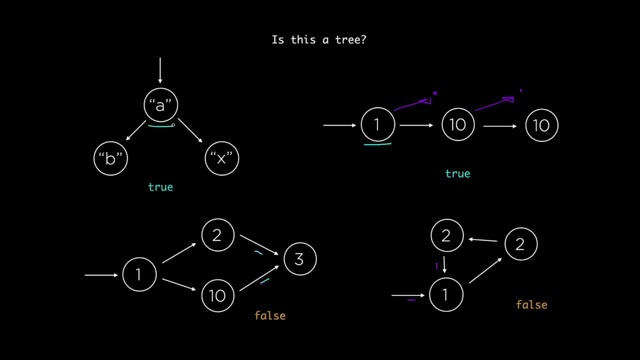 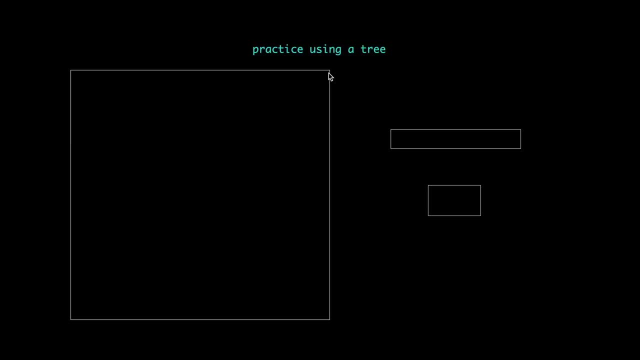 no other node refers to that one. Okay, now that you hopefully have a clear idea of what a tree is, let's practice using a tree. with this problem, You're given a tree, for example this one, with the root being here: 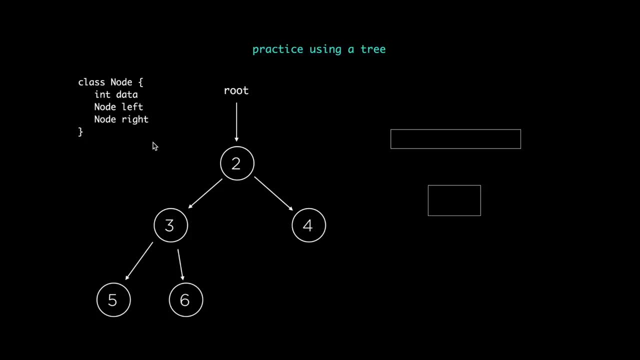 And this is a binary tree, So the class of each node will look like this: It has an integer of data And it has two children left and right, And the problem is writing a function which we're going to call findSum. 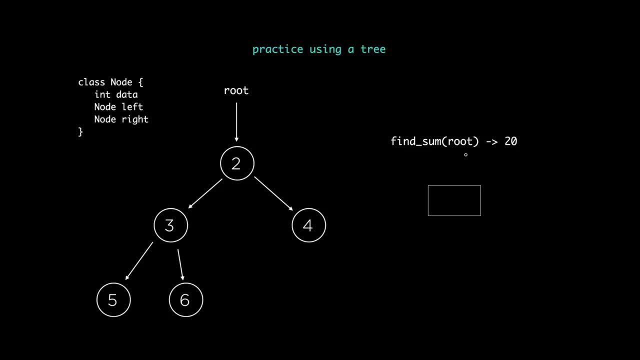 which takes the root of this tree as the input and returns the sum of all the values within this tree. So if you're given this particular root, you want to be able to return 20 from this function, because we have 2 plus 3 plus 5 plus 6 plus 4,. 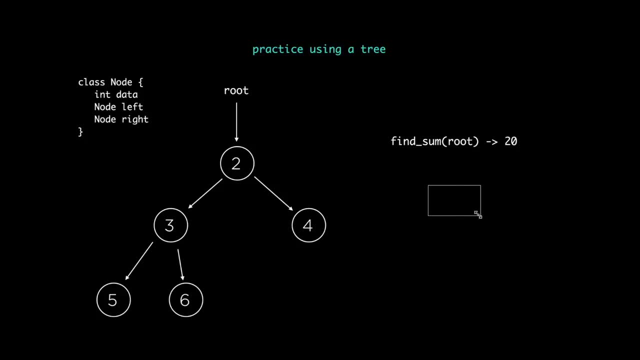 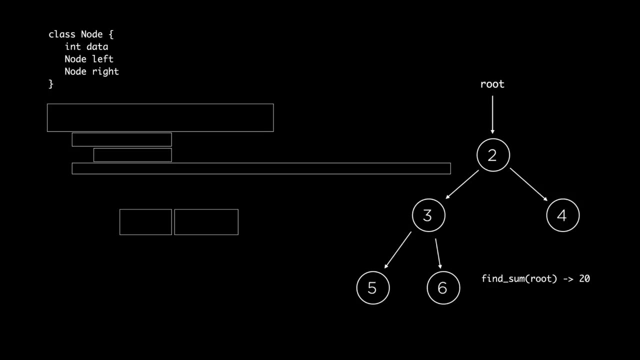 which is 20.. And try solving this problem In O of n in time, where n is the number of nodes in this tree. Okay, and here's my solution. And, by the way, if you want to try running my solution in either Python or Java, 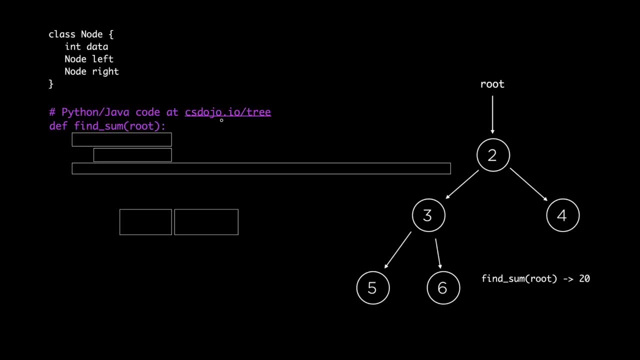 you can find that at this URL: cssocialio slash tree. Like I said before, we're calling this function findSum and it's taking the root of whatever tree that you're given And we're going to implement this function recursively here. 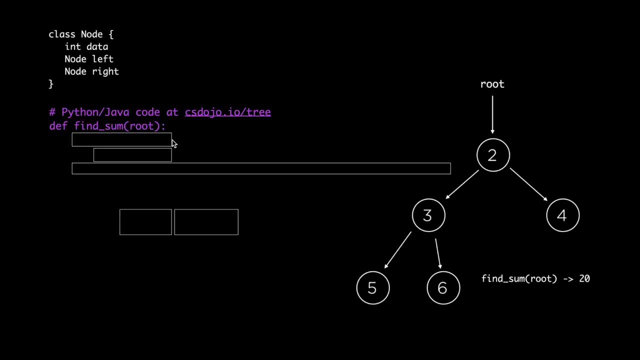 And the first thing we're going to do is we're going to define the base case, And that's going to be when the given root is null or none, which is that the given root is just an empty tree, For example, this empty tree right here. 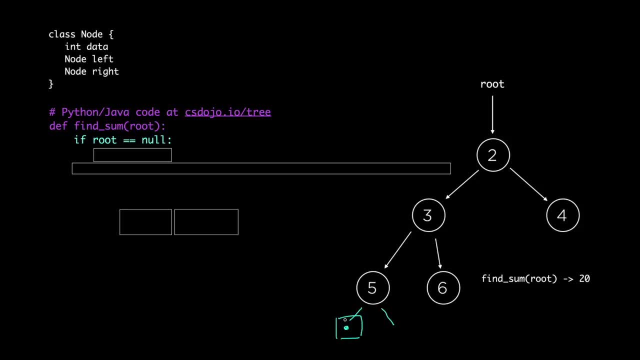 Then the sum of all the values in this empty tree is of course 0. So we want to return 0 in that case. And otherwise, for example, if we're given this root right here in this recursive function, then the sum of all the nodes in this tree. 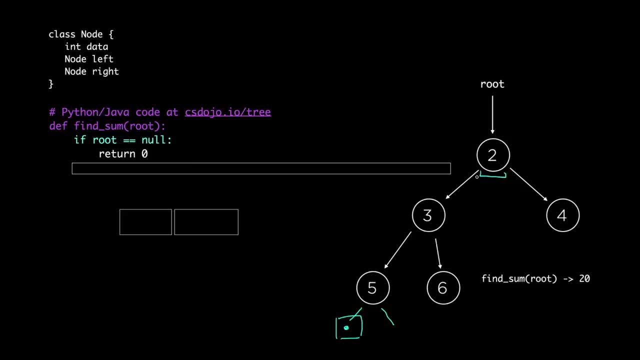 is the sum of this current value plus the sum of all the nodes in the right subtree and the sum of all the nodes in the left subtree. We can express that with this one line here We're returning the current value, or rootdata. 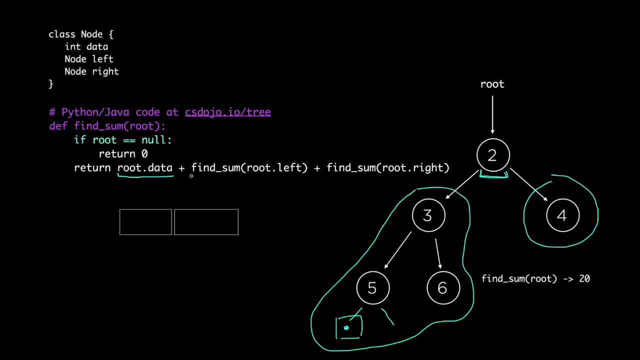 plus the sum of all the nodes in the left subtree, So that's findSum of rootleft, and the sum of all the nodes in the right subtree, So that's findSum of rootright. And this function would only take O in time to execute. 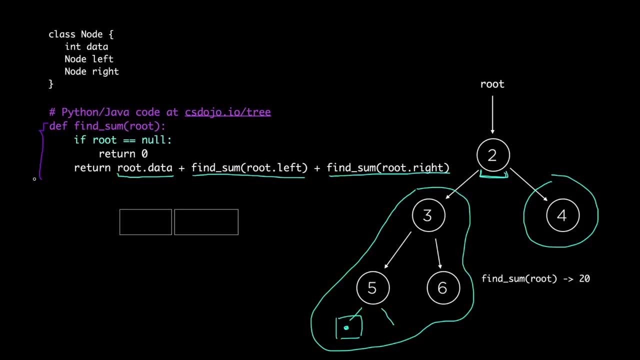 where n is the number of nodes in the given tree. And let's think about why. Well, first we need to count the number of times this function is going to be called, And that's going to be the number of nodes in the given tree. 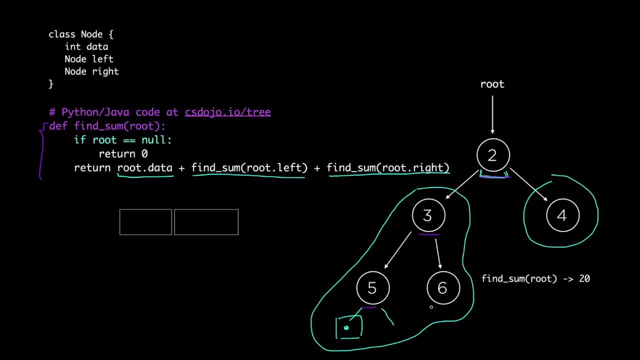 because for each node this function is going to be called once, plus all the empty nodes or these empty trees that I didn't draw earlier in this representation of the tree, And so this function is going to be called at most about 2n times. 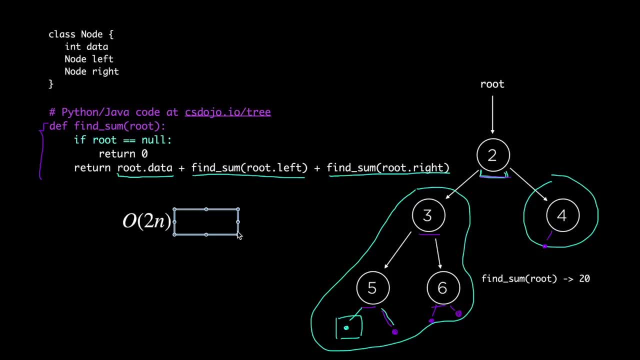 or O, which is the same thing as O, And so this function is going to be called O, and each time this function is called, let's think about how much time it takes to execute. Well, if you look at each line,